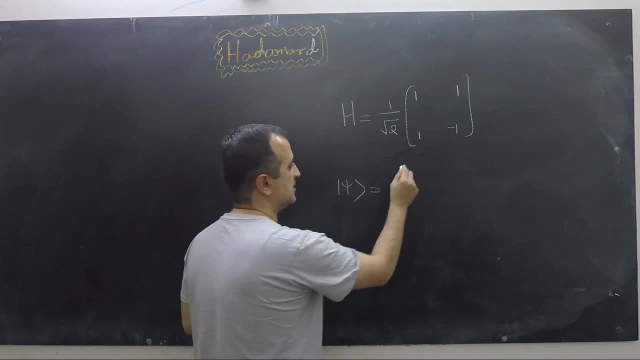 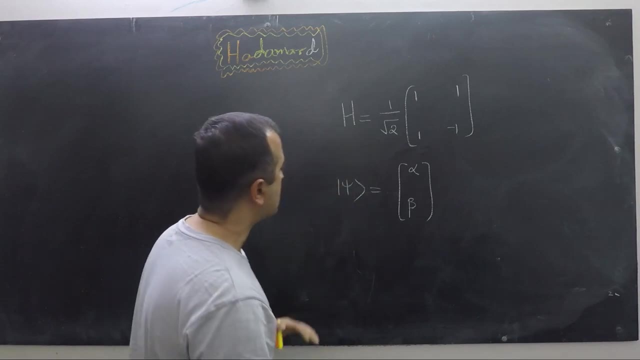 can be expressed as a vector which is alpha and beta, Where alpha and beta are complex numbers. So we can apply Hadamard gate on this qubit by simply multiplying Hadamard gate, Hadamard gate with cat psi and we have our transform qubit cat psi bar. 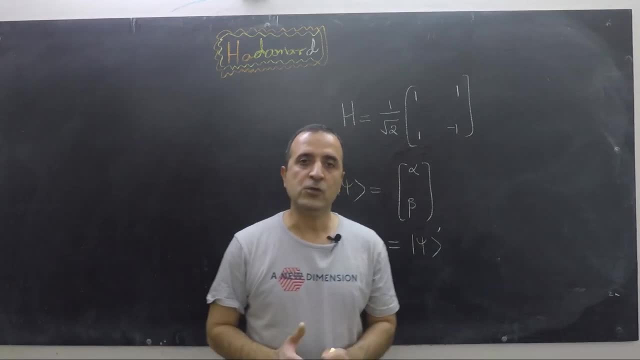 A key use of Hadamard gate is that you give input a qubit in pure state and Hadamard gate create a qubit in equal superposition. So let's understand it with some examples. So let's say I have a Hadamard gate. 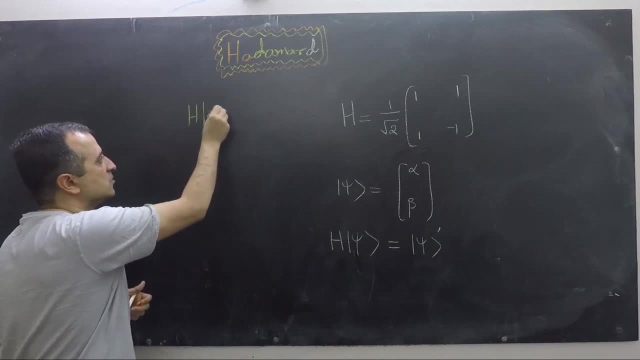 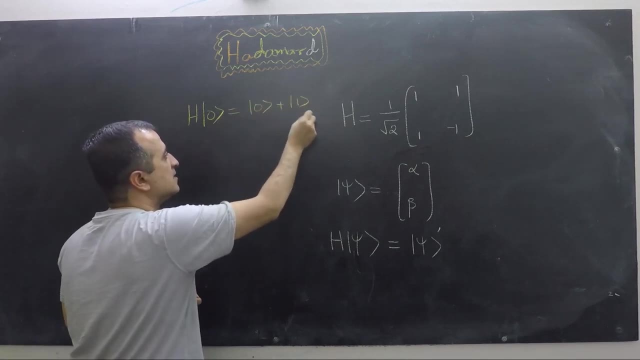 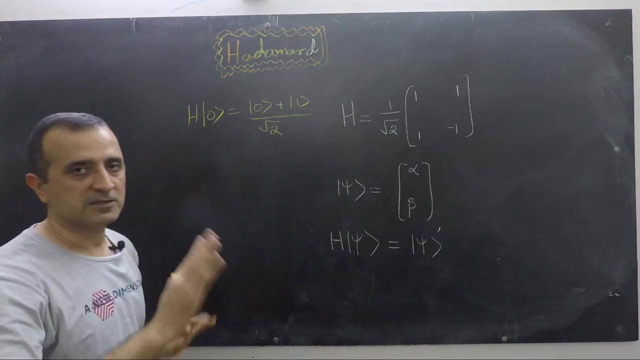 And I apply that Hadamard gate on cat 0. Then my answer is going to be cat 0 plus cat 1 divided by square root of 2.. That means in this case my probability of getting 0 was 1.. So it is a pure state Where this is a equal superposition. That means I can get. 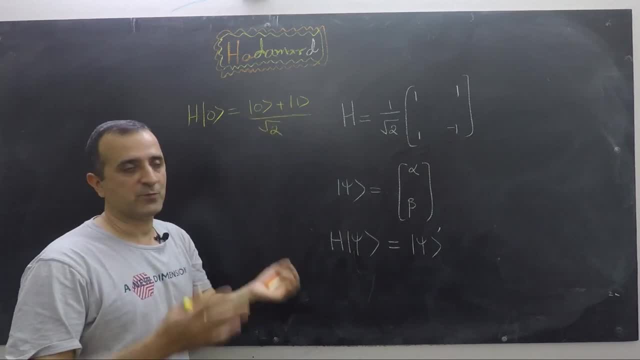 either 0 and 1 with same probability. with 0.5 probability I can get 0. with 0.5 probability, I can get 2. with 0.5 probability, I can get 3 with 0.5 probability. 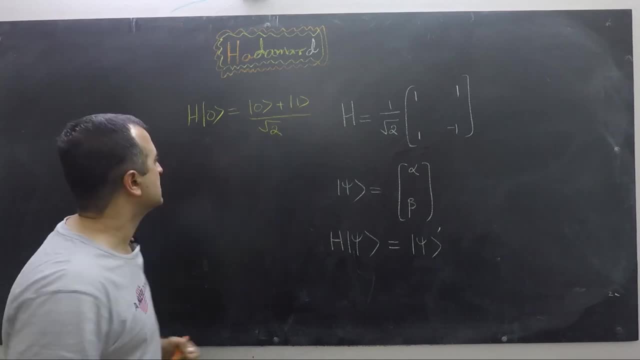 I can get 4 with 0.5 probability. I can get 5 with 0.5 probability. I can get 4 with 0.5, 1 with 0.5 probability. Similarly, if we give Hadamard gate another qubit, let's say ket 1,. 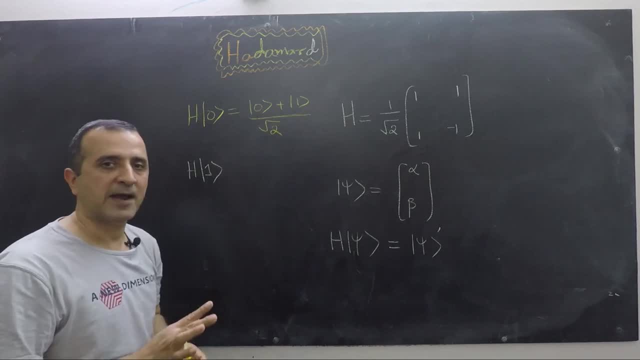 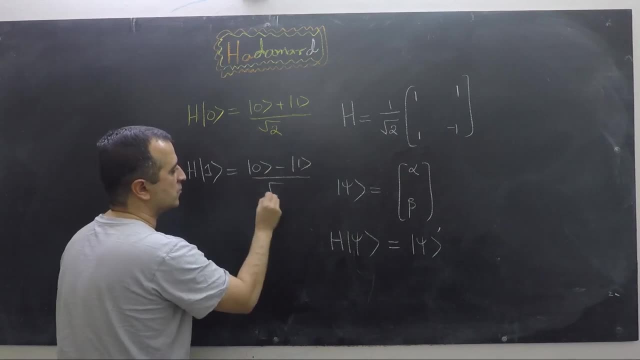 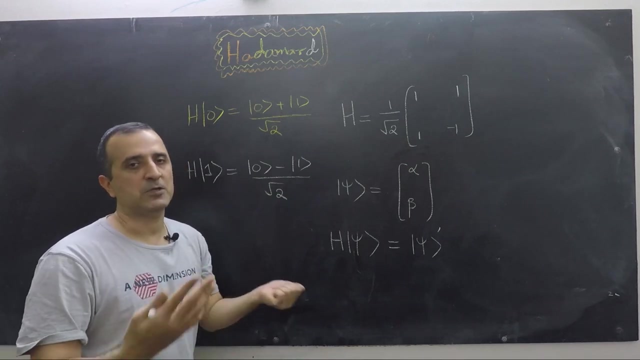 we will once again get equal superposition, but there might be some phase shift. So we'll get like ket 0 minus ket 1 divided by square root of 2.. But this minus sign does not change probabilities, because probabilities are square of amplitude and minus sign are illuminated when we square. 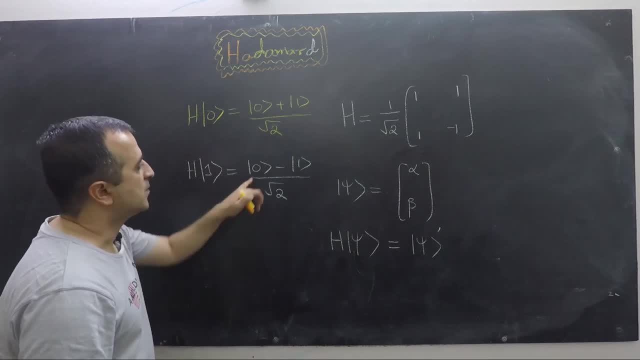 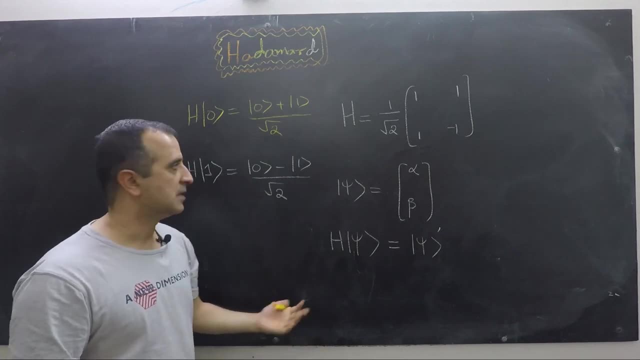 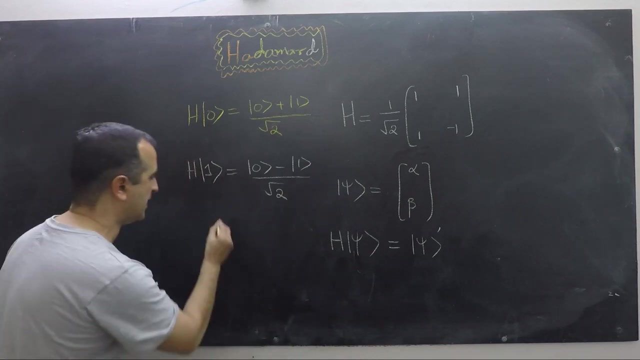 the amplitude. So in this case also, the probability of ket 0 is 0.5 and probability of ket 1 is also 0.5.. So Hadamard gate takes input of pure state and create equal superposition. Let me write it down. 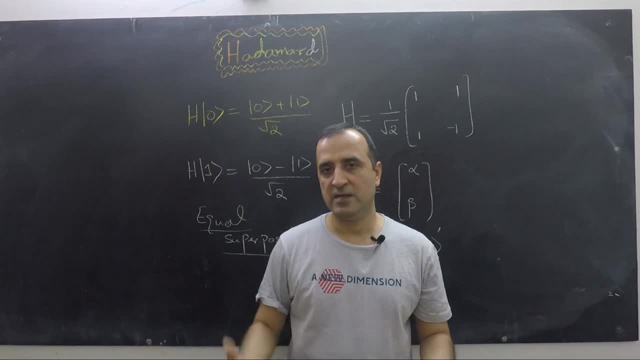 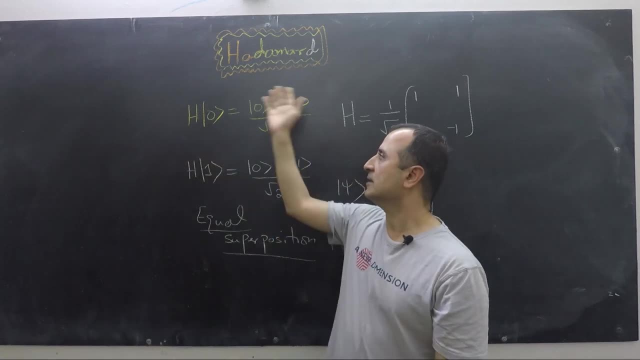 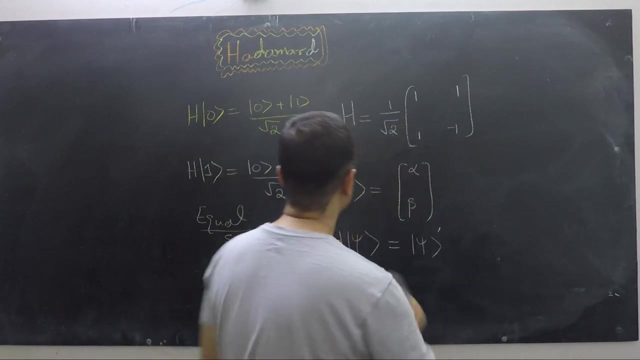 My goal of this video is to explain everything clearly. So instead of just saying that Hadamard gate is applied on ket 0, we get this result. I want to show that this result is indeed correct. So let's see that Now. this is very easy and simple to understand. 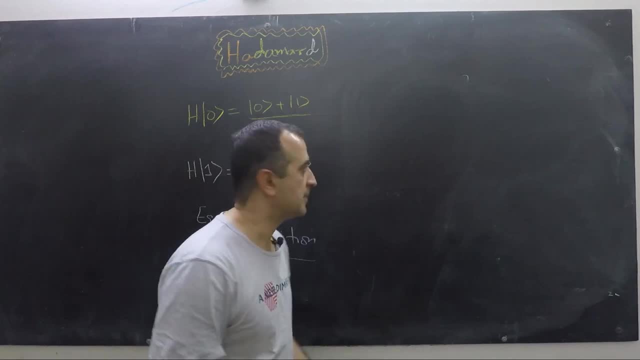 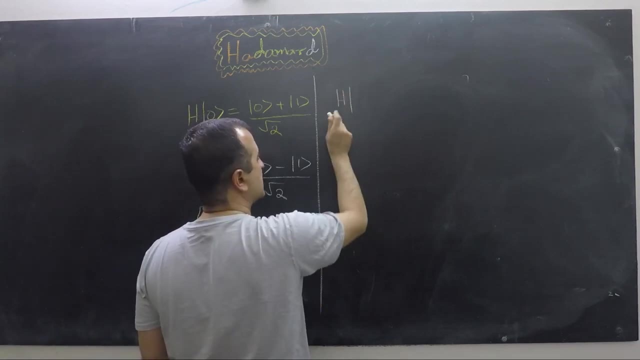 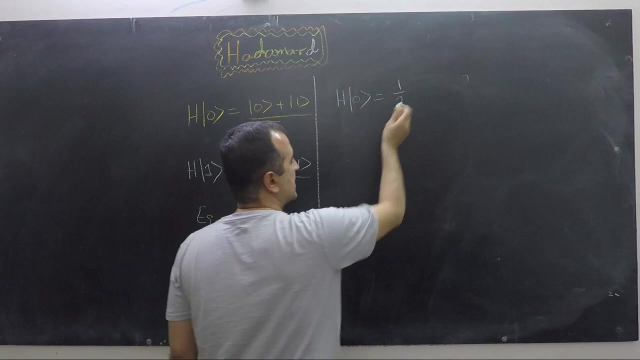 but I have to show it for everyone so that everyone can understand. We are all on the same page. So I apply Hadamard gate on ket 0. This is basically multiplying this matrix. that matrix represents Hadamard gate with this vector, And this vector, ket 0, is expressed as: 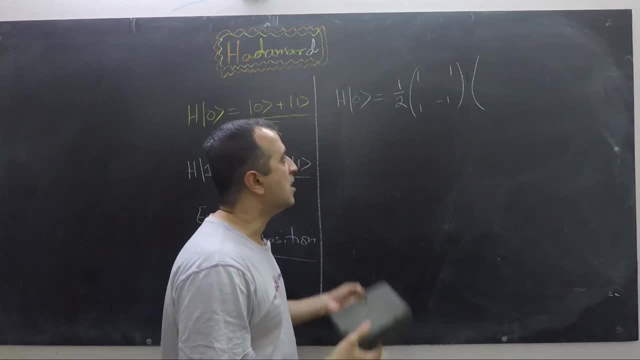 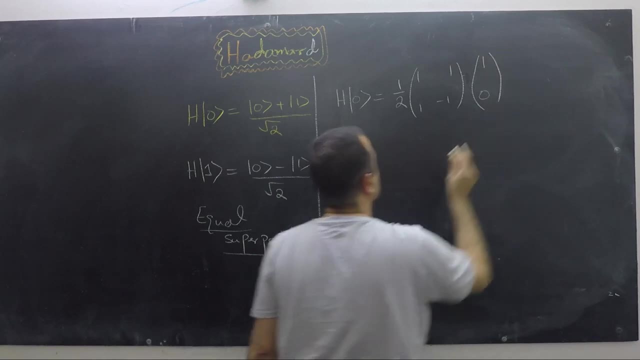 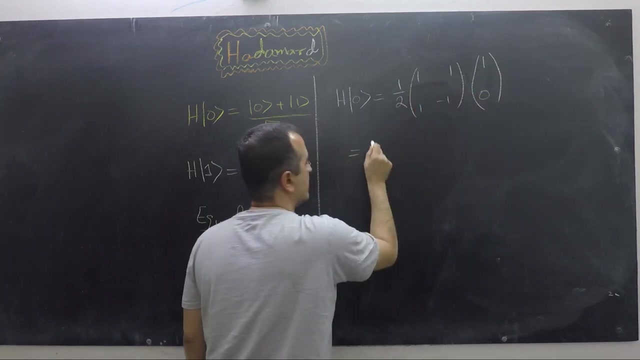 a vector whose zeroth location has 1 and all other locations has 0. So zeroth location has 1 and other location has 0. Now we multiply this matrix with this. We get here 1 over square root of 2.. By the way, it should be square root of 2. But we get 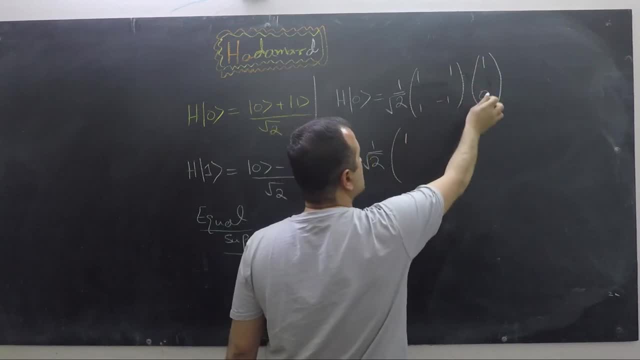 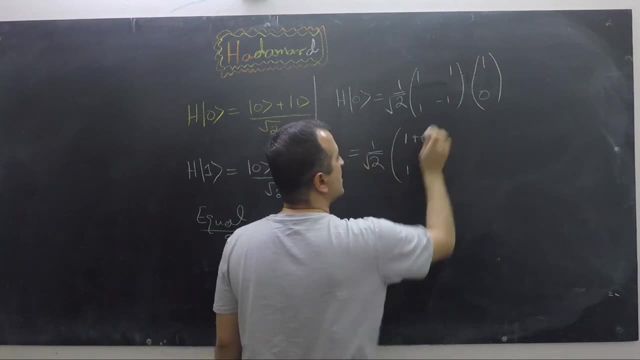 1 multiplied by 1 is 1.. 1 multiplied by 0 is 0.. And then we multiply this by this: We get 1 multiplied by 1 is 1.. And minus 1 multiplied by 0 is 0.. And then we simplify it: We get 1. 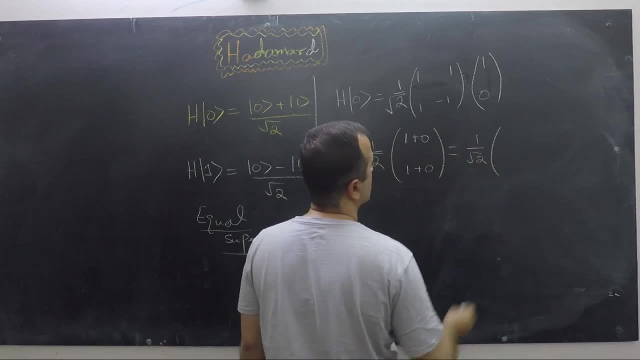 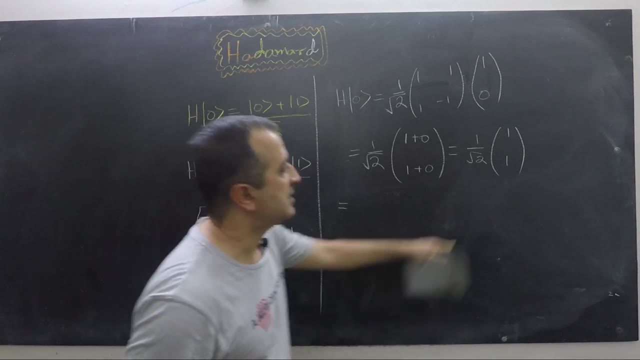 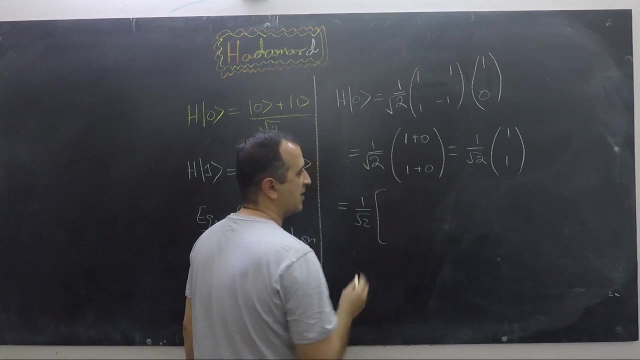 over square root of 2.. We have here 1: 1.. Now we can write this result in two different vectors. We can write it like this: 1 over square root of 2.. And I can write here: ket 0, which is 1: 0.. And I can write: 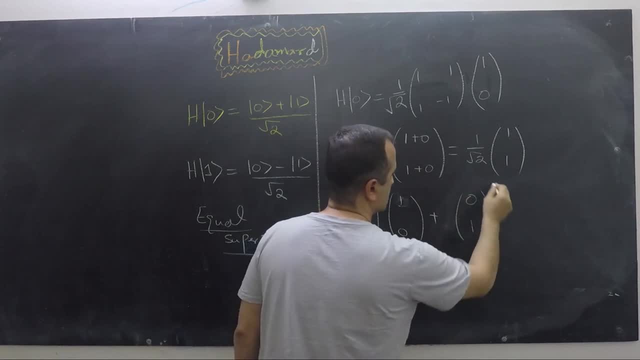 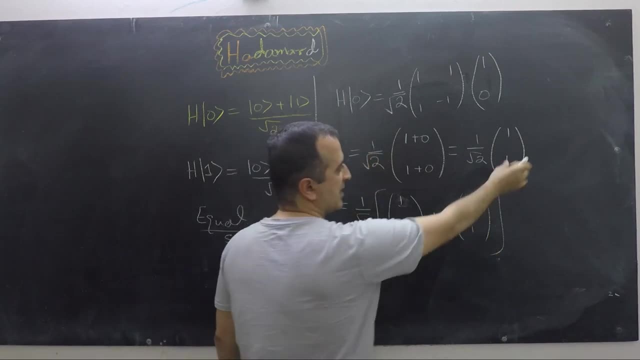 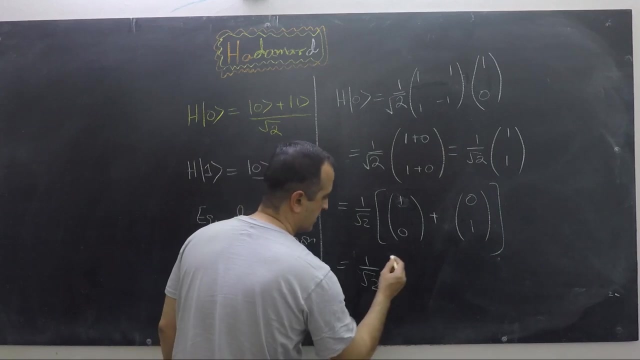 it as ket 1, which is 0, 1.. So this vector here represents ket 0.. This vector here represents ket 1.. And if I add both of those vectors get this result. so then this simplifies to 1 over square root of 2. I have here: 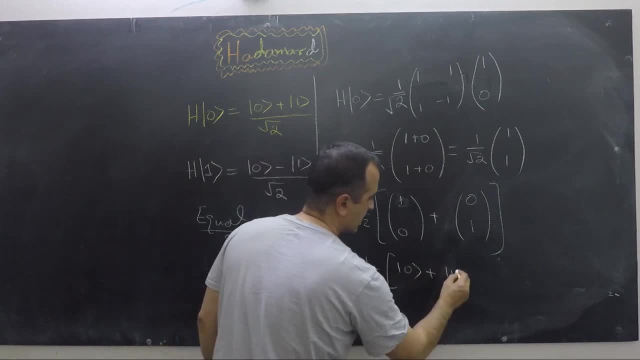 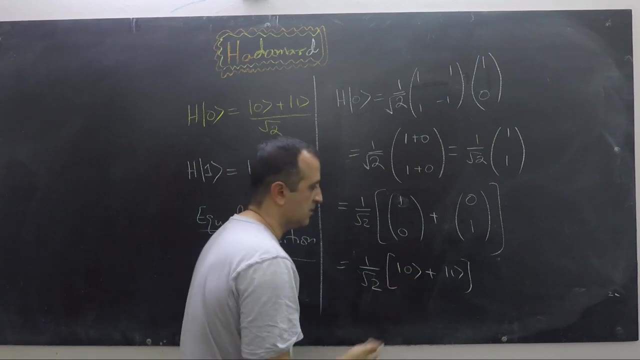 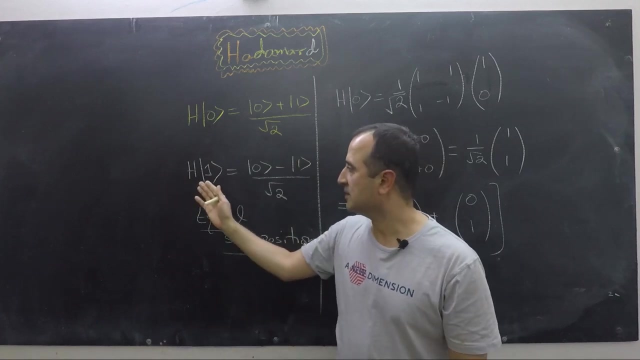 cat 0 plus cat 1, or I can simply take 1 over square root of 2, underneath it in the in the denominator for same thing. so I have shown that this result was indeed correct. similarly, you can yourself try this out- that this is also correct only. 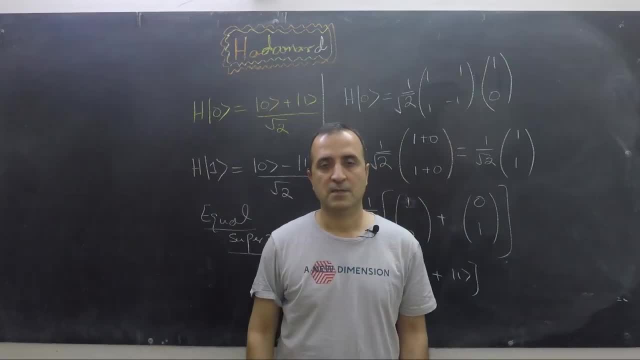 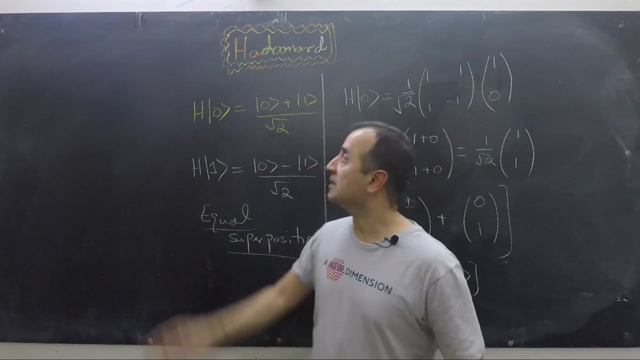 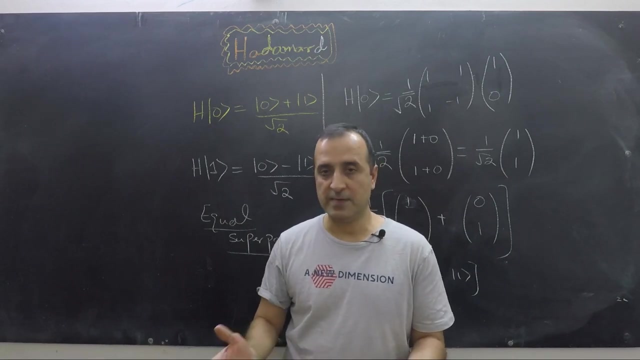 changes the sign here, as I have explained earlier, that all quantum gates are unitary. the all quantum gates must be unitary, but there are many quantum gates which are also hermitian. Hadamard gate is one of those quantum gates which are both unitary and hermitian. let's recall what that means. so for unitary. 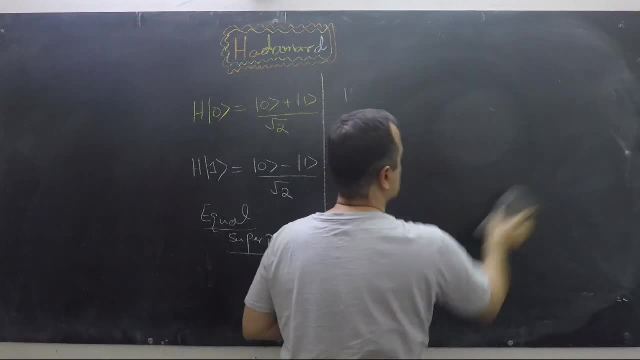 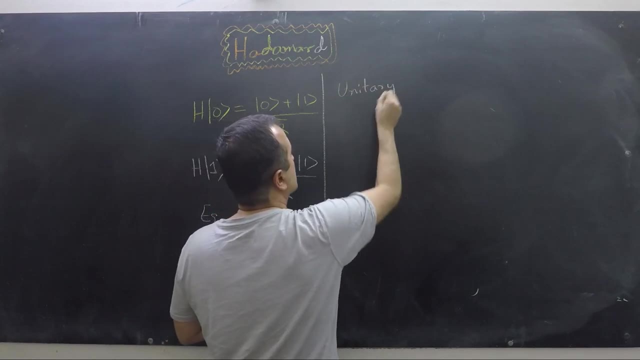 gate, we say, is that its inverse is equal to conjugate transpose. so let's say so: Hadamard is unitary gate. so we can say Hadamard gate multiplied by conjugate transpose is equal to identity. that's the definition of unitary. so basically, inverse of Hadamard gate is equal to its conjugate transpose. and what is conjugate transpose is that you take, transpose and also you change sign of all the terms that have identified it. and another thing is this: that Hatam scr Wing is also hermitian. 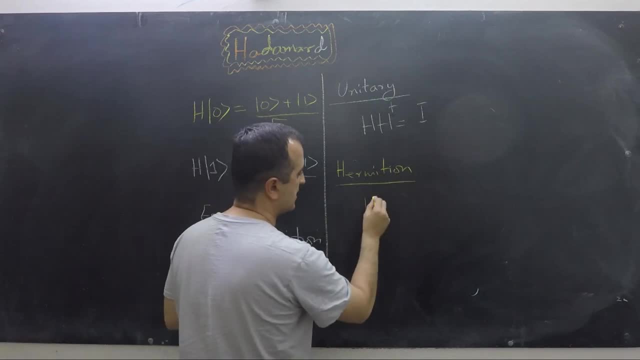 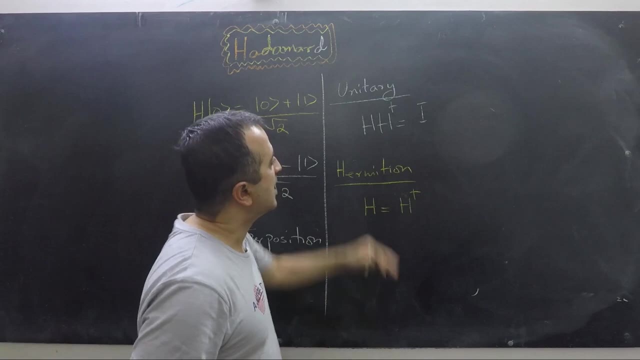 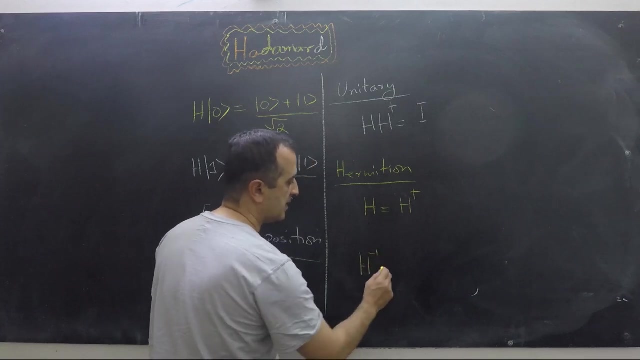 Term hatemart gate emplies that Hatemart gate is equal to conjugate transpose. so Hadamard gate is equal to conjugate transpose and if you combine both of those then we can write that inverse of Hadamard gate is basically Hadamard gate. We don't have to take conjugate transpose, we can just say: 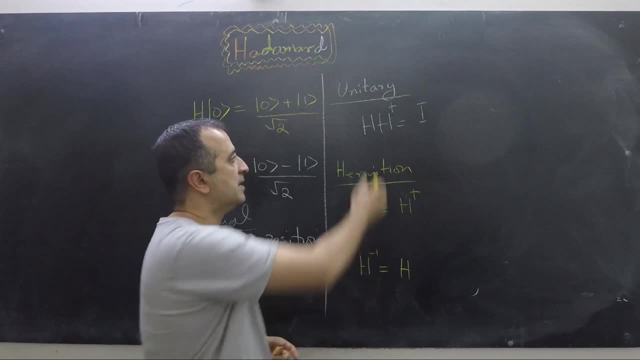 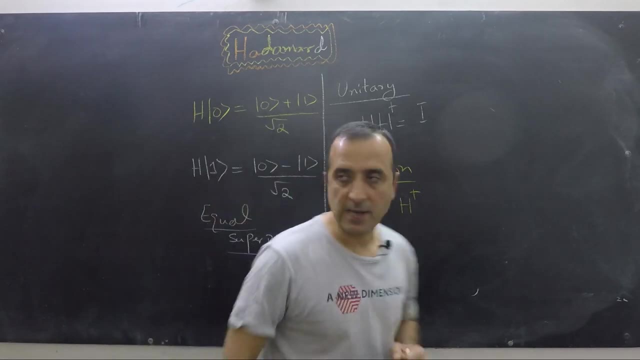 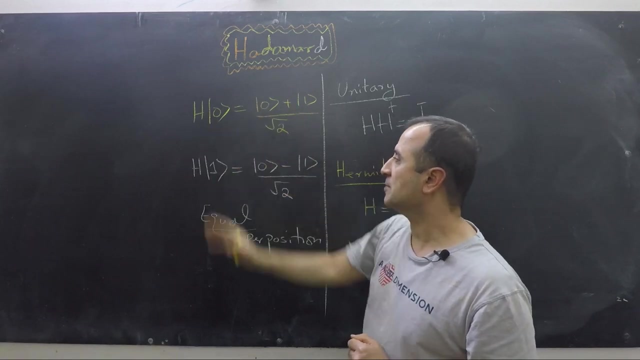 inverse of Hadamard gate is Hadamard gate by combining both of them. If this statement here is correct, then if I apply Hadamard gate on equals proposition of ket 0 and ket 1, I should get 0. Similarly, if I apply Hadamard gate on this: 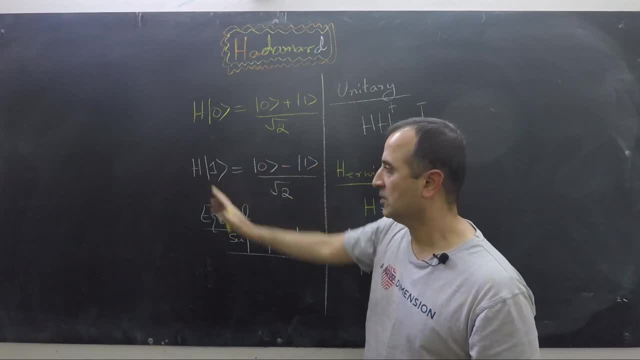 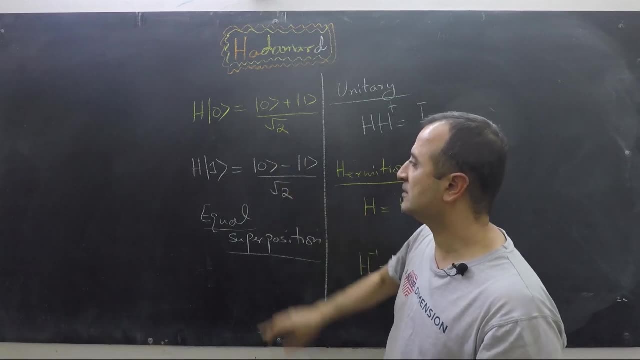 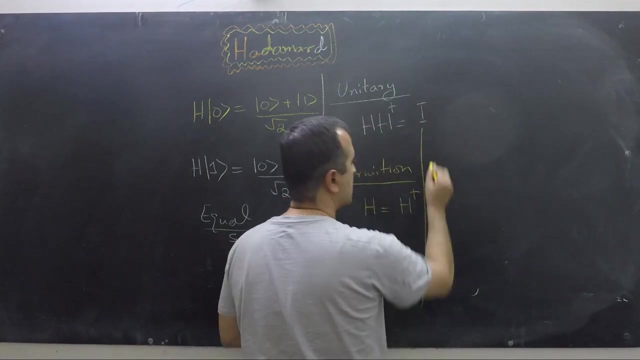 equals proposition of ket 0 and ket 1, I should get ket 1.. So let's try it, and if Hadamard gate is inverse of itself or not, so we apply Hadamard gate on this thing and see if we can get ket 1 or not. So we apply Hadamard gate on this one. 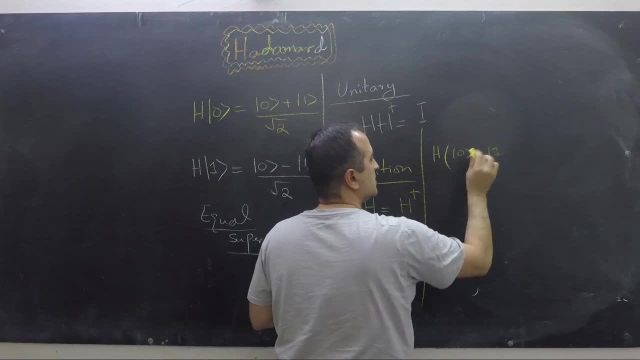 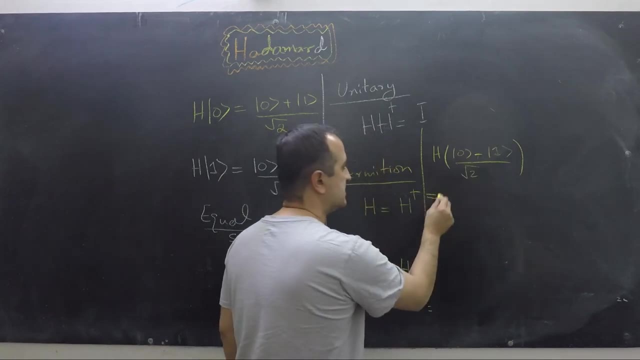 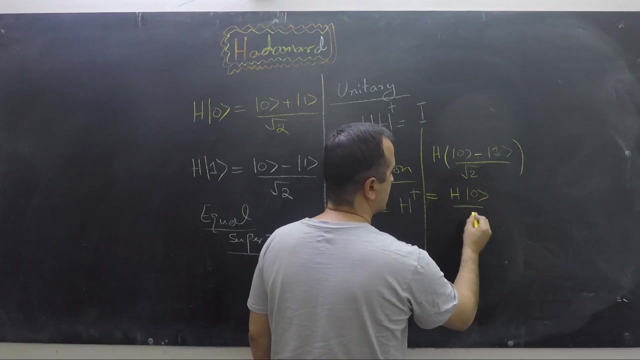 which is ket 0 minus ket 1 divided by square root of 2, and this is same as saying that I apply Hadamard gate on this thing. So if I apply Hadamard gate on Hadamard gate on cat 0 divided by square root of 2, and I apply Hadamard gate on cat 1,